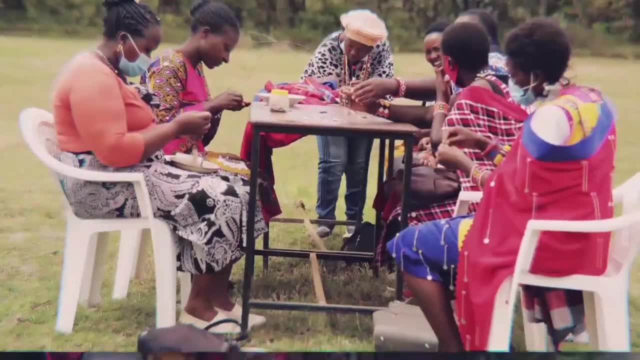 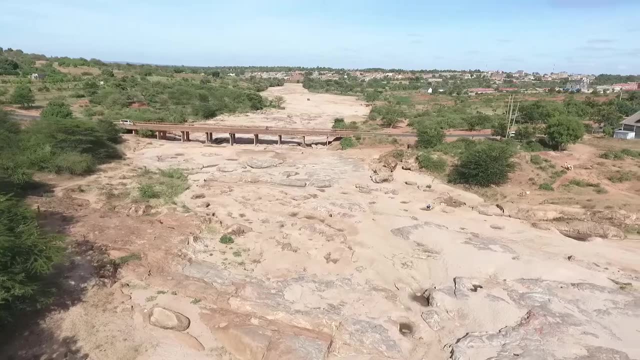 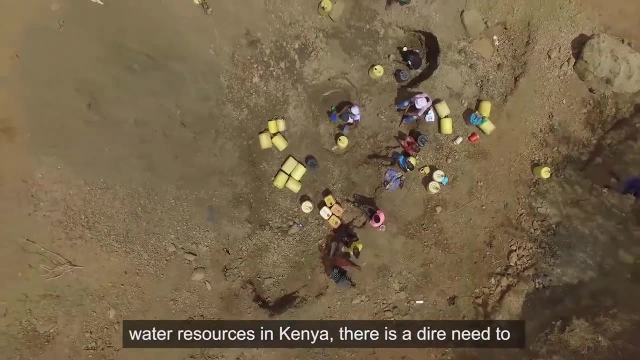 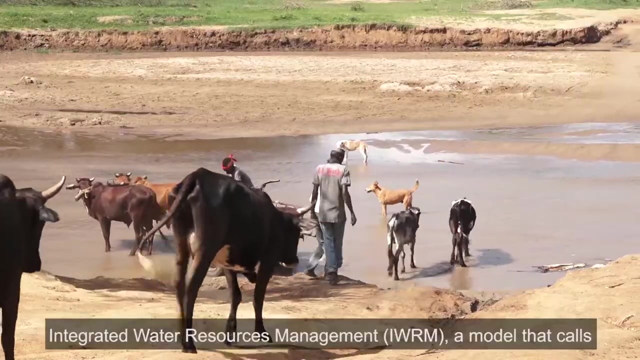 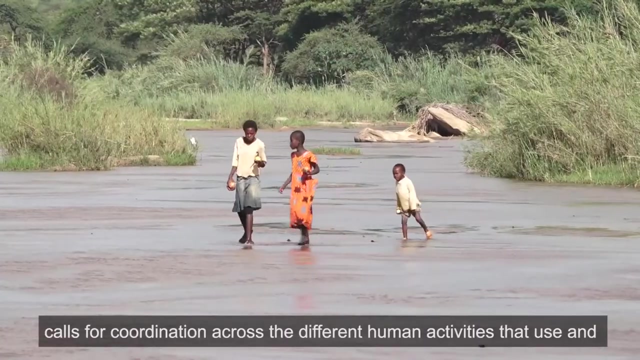 As climate change continues to strain the already limited water resources in Kenya, there is a dire need to conserve and manage what is left properly Integrated Water Resources Management- IWRM- a model that calls for coordination across the different human activities that use and affect water in a river basin. 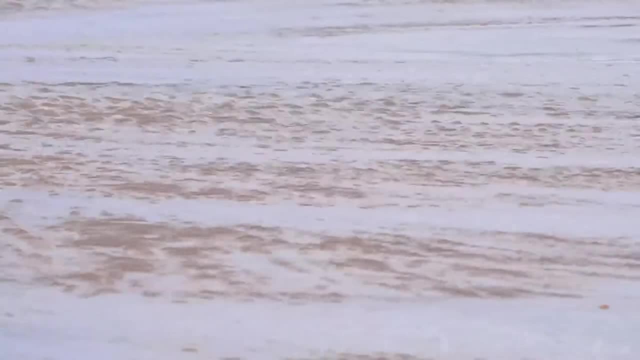 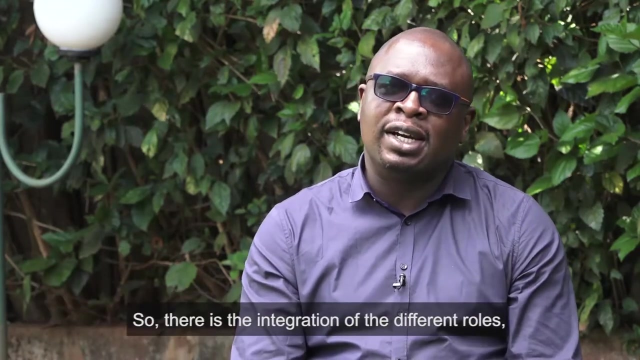 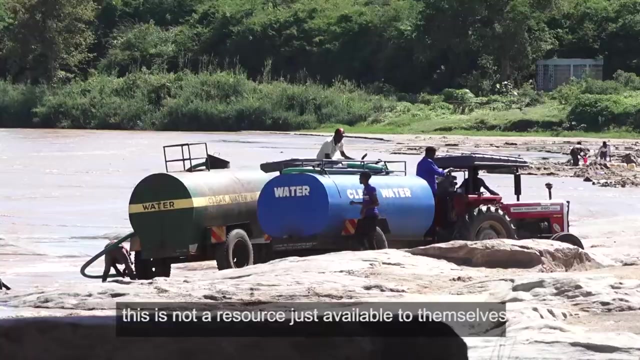 could be the solution to water crisis in the country. IWRM also really depends on a cooperative engagement. So there is the integration of the different roles of different partners, cognizant of the fact that this is a resource that is not just available to themselves. 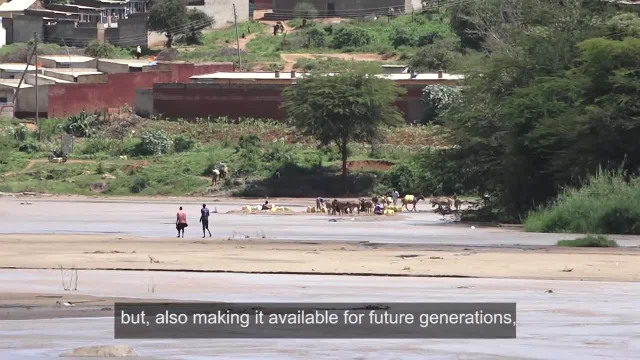 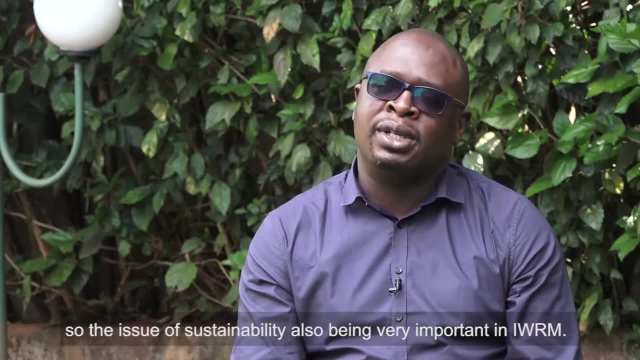 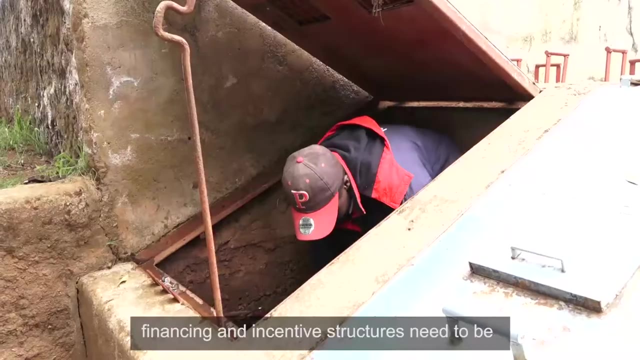 but also needs to be there to other users, but also making it available for future generations. So the issue of sustainability also being very important in IWRM. For IWRM to be effective in a river basin, financing and incentive structures need to be established. 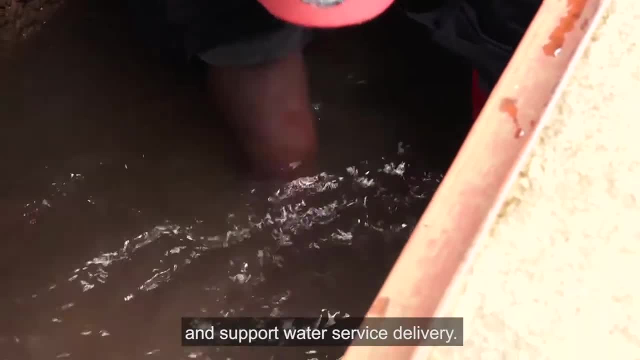 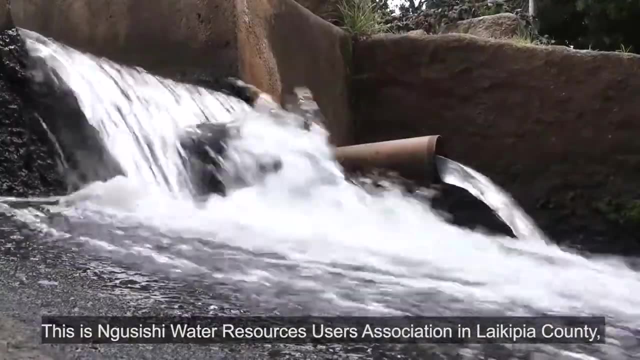 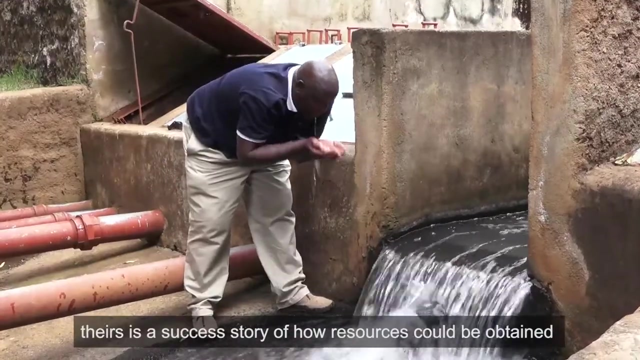 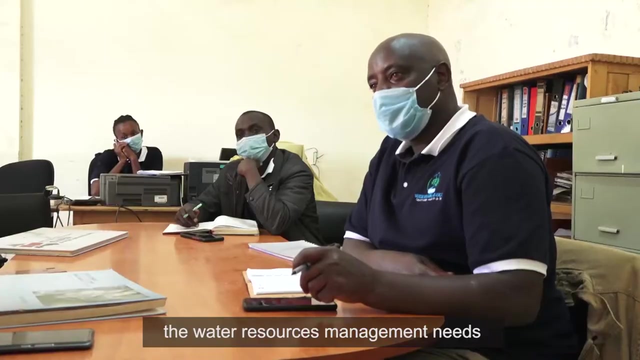 to fund capital-intensive water projects and support water service delivery. This is Ngosese Water Resources Users Association in Laikipe County. Theirs is a success story of how resources could be obtained from private finance or public-private partnership since the government may not be able to meet all the water resources management needs. 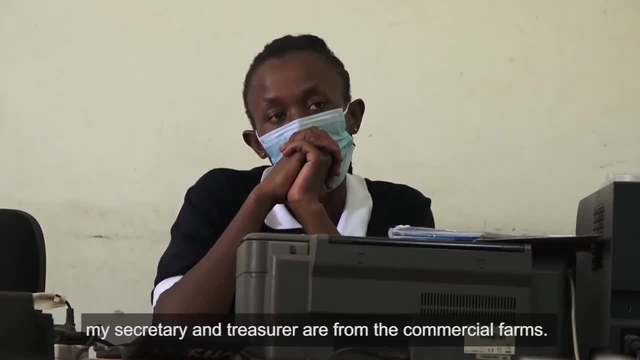 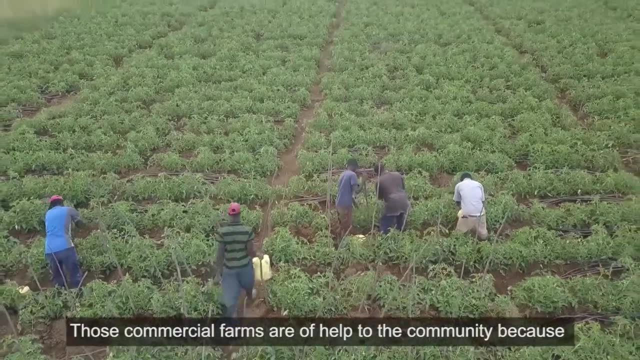 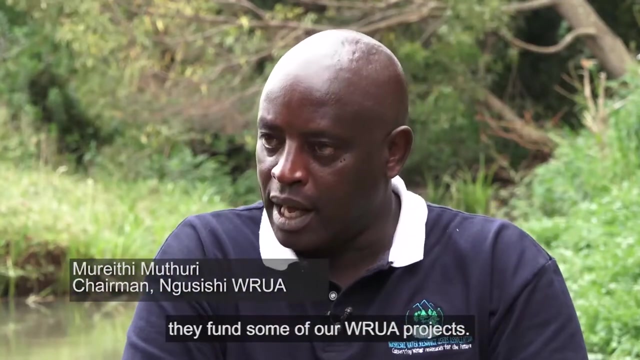 We sit down together, my secretary and treasurer are from the commercial farms And if those commercial farms are of help to our communities, because most of the project funding, some of the ritual funding, they fund the river, Some activities where we can identify an activity. 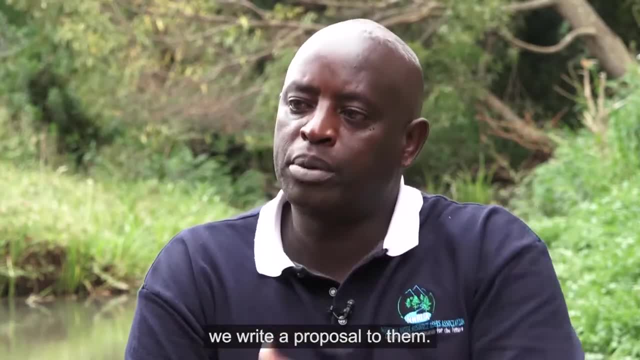 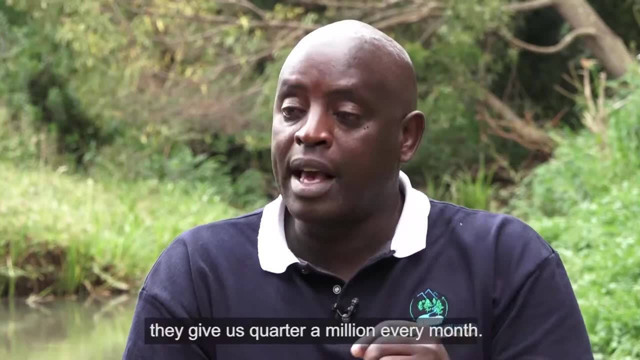 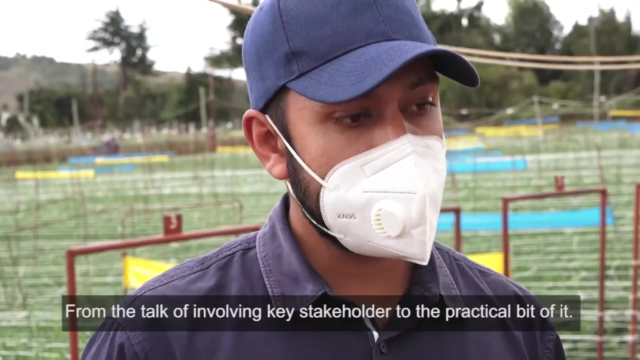 if it is less than a million, we write a proposal to them and they fund. We have one good farm like Timafro. they give us a quarter million every month. From the talk of involving key stakeholders to the practical bit of it. 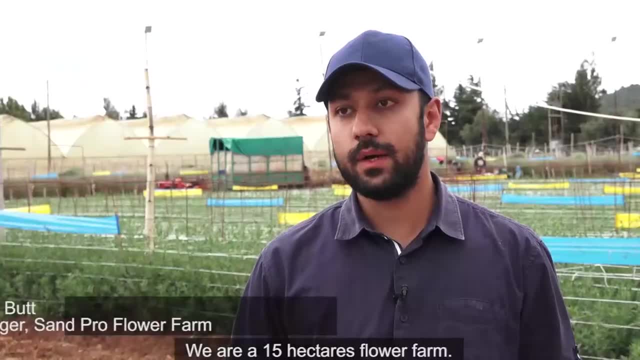 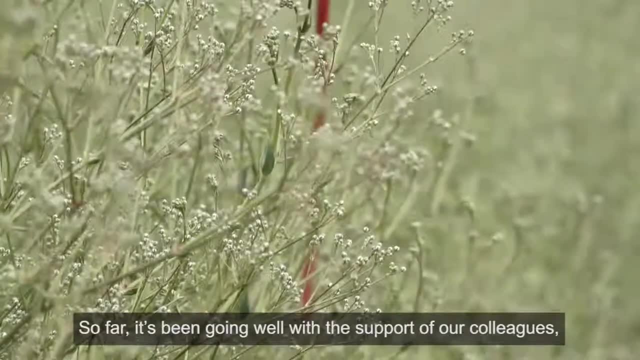 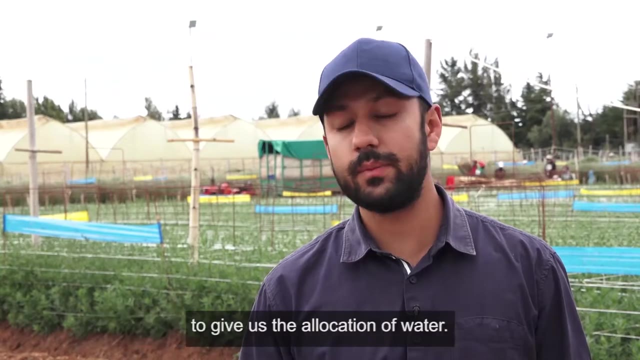 Ngosese is walking the talk. We are a flower farm, 15 hectares. so far it's been going well with the support of our colleagues, Ngosese Water Resources, who have been very good to us being able to give us allocation of water. 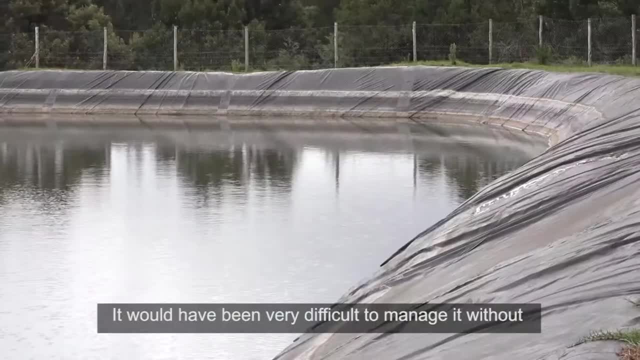 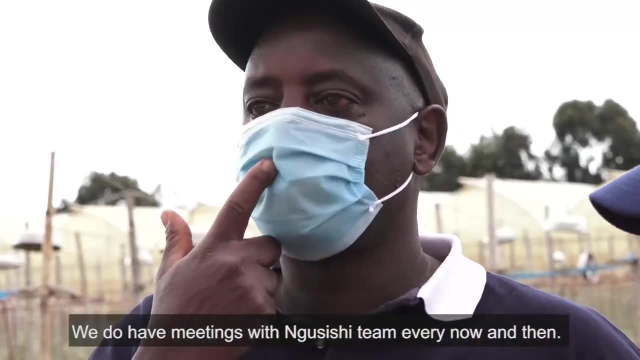 So it would have been very difficult to manage it without the allocation. from the spring. We do have meetings with the Ngosese team every now and then and we do help each other as a team, especially when we have to maintain the line. 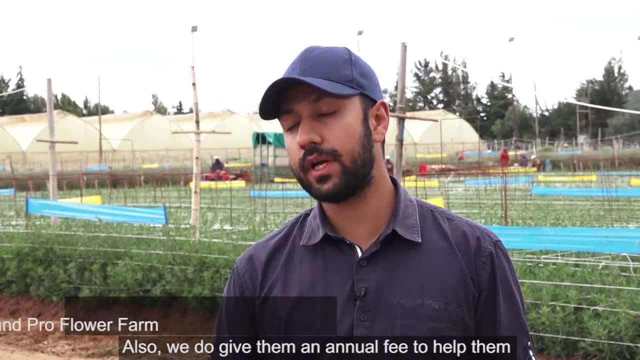 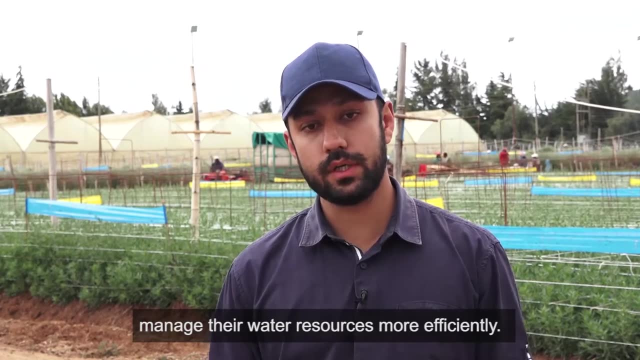 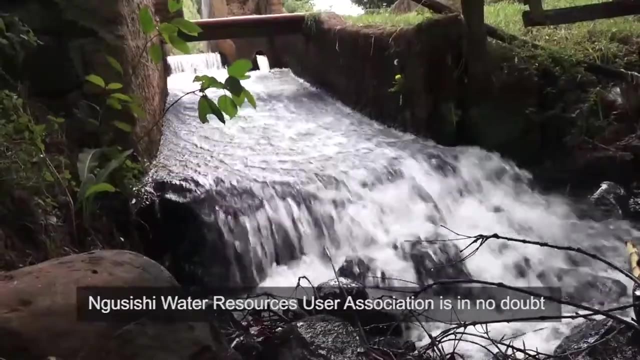 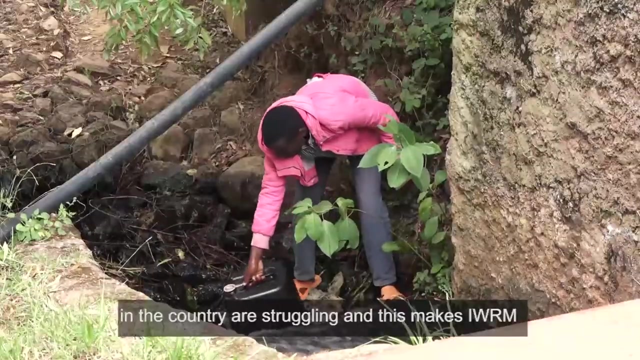 Also, we do give an annual fee to Ngosese Water Resources every year, which helps them also manage the water resources more efficiently. Ngosese Water Resources User Association is in no doubt a success story, but most of the water resources users associations in the country are struggling. 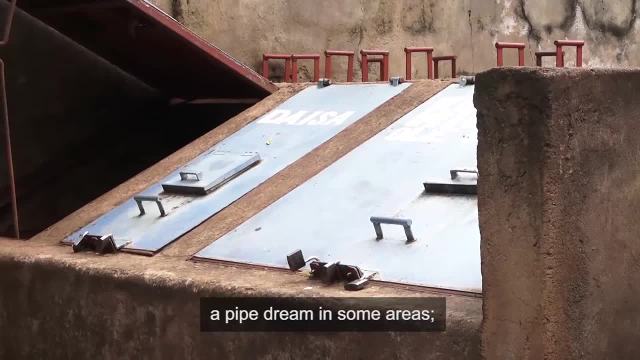 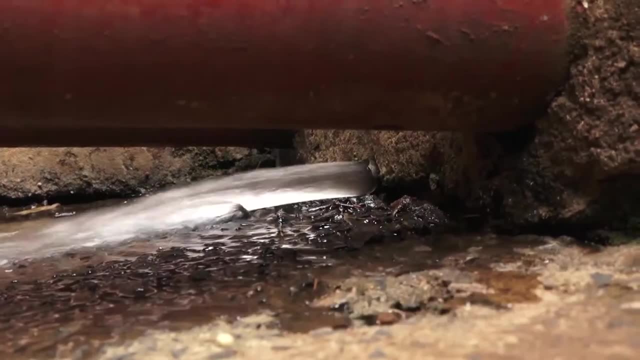 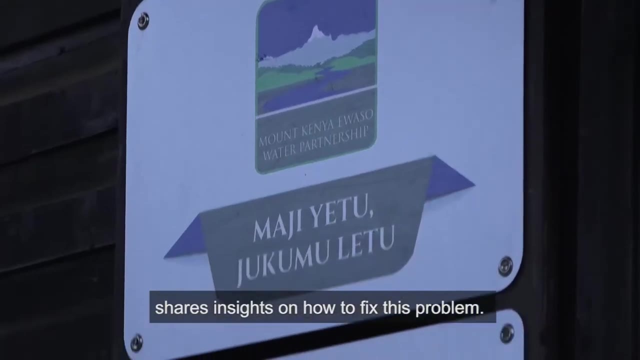 and this makes IWRM a pipe dream in some areas. Ngosese is under Mount Kenya Iwaso Water Partnership. Stanley Kirimi, the coordinator of Iwaso Water Partnership, shares insights on how to fix this problem. So what we have come up with is a cooperative. 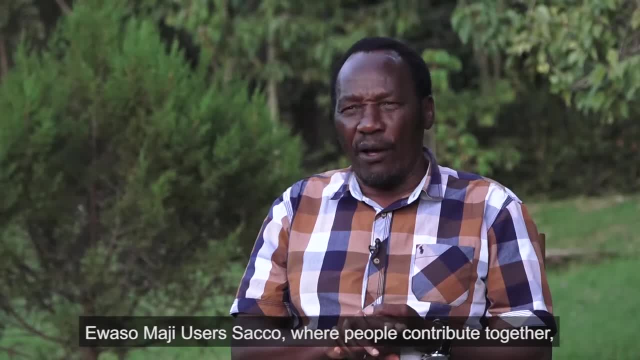 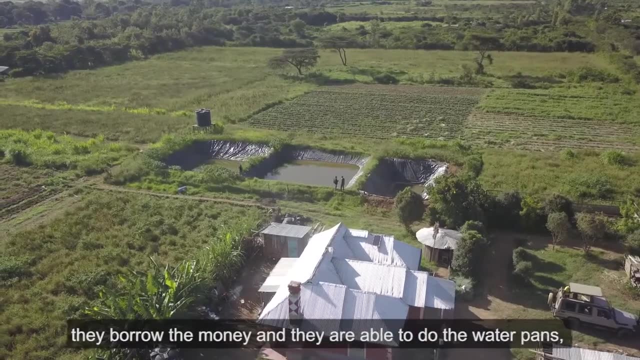 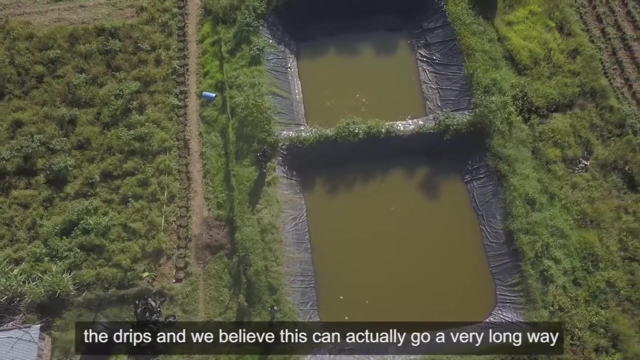 water, a cooperative called Iwaso Merge Users Circle where people contribute together, they borrow the money, they are able to do the, the water pans, they are able to do the drips, and we believe this can actually go a very far way. 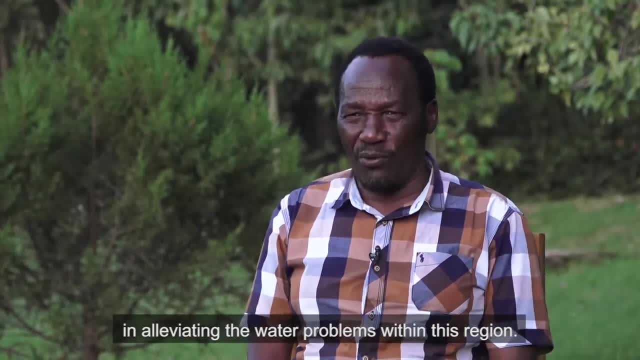 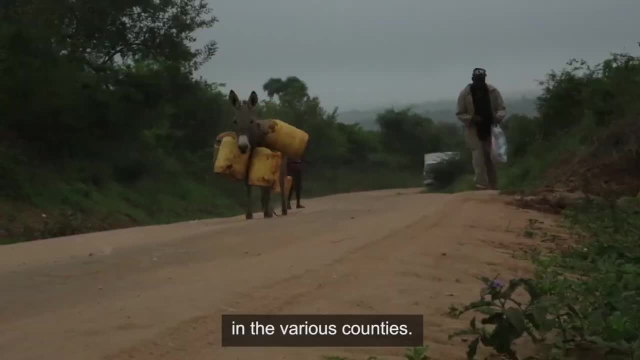 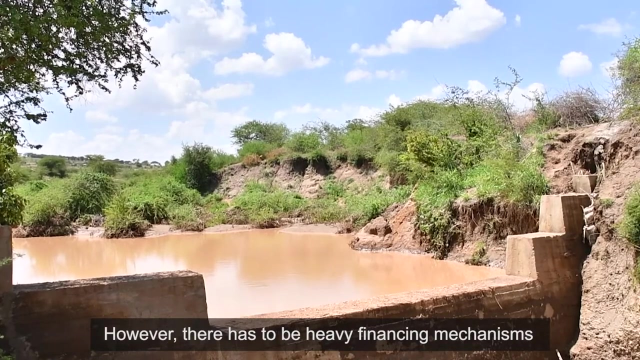 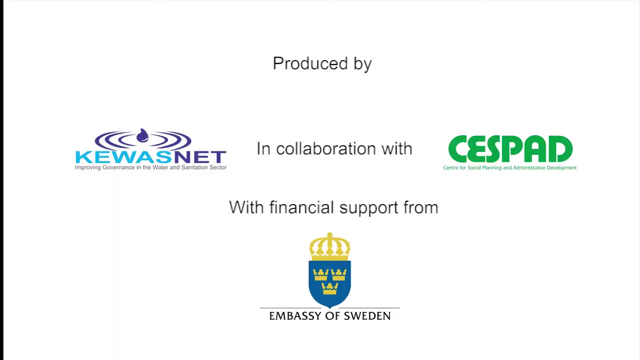 in alleviating the problems of water within this region. IWRM is a model that will ensure efficient water governance in the various counties. However, there has to be heavy financing mechanisms for the model to work effectively. IWRM is a model that will ensure efficient water governance in the various counties.